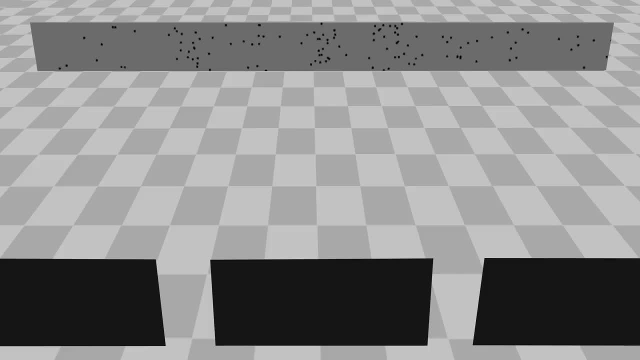 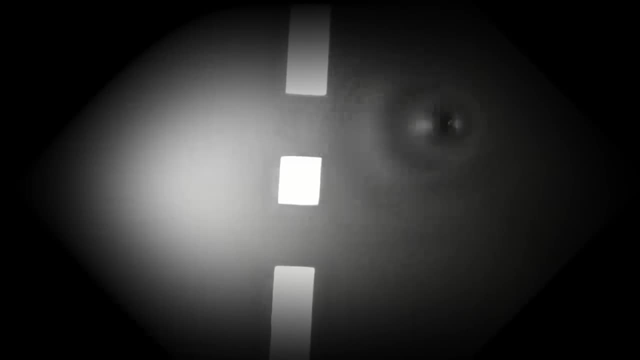 they produce an interference pattern Even when you send each electron through one at a time. With walking droplets, the pilot wave goes through both slits, interfering with itself, while the droplet only goes through one slit. The droplet doesn't move in a straight line, though. 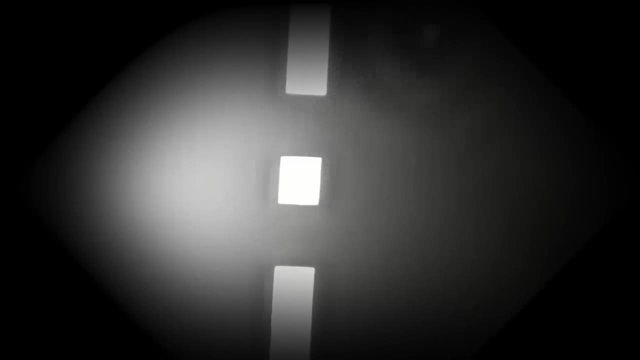 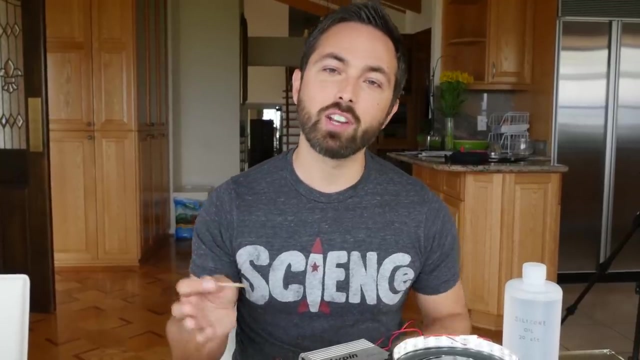 It's deflected by its interaction with the wave. The resulting distribution of where the droplets end up looks very similar to quantum double slit interference patterns. Or take tunneling. In quantum mechanics it's possible for a particle to get through a barrier. 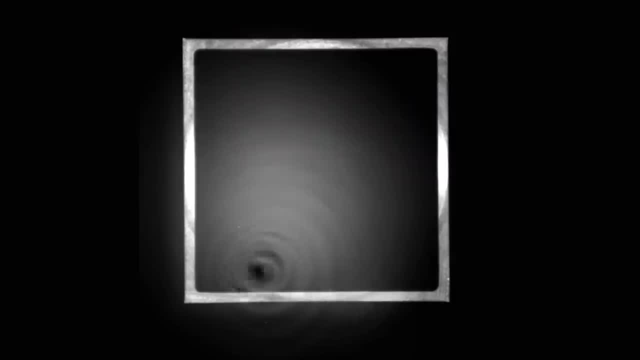 that it wouldn't classically have enough energy to get over. This has been demonstrated with walkers by creating a shallow barrier under the surface of the oil. Usually, the barrier reflects the pilot wave and its bouncing droplet, But in rare cases the droplet does cross the boundary. 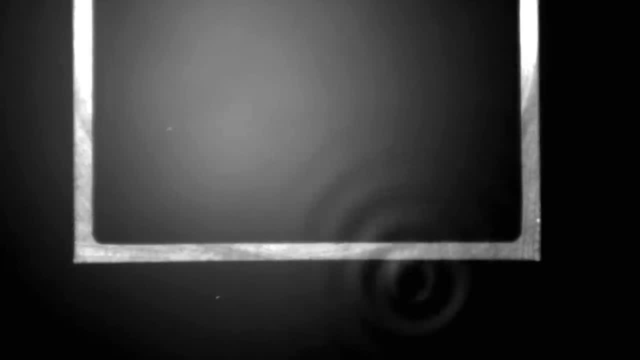 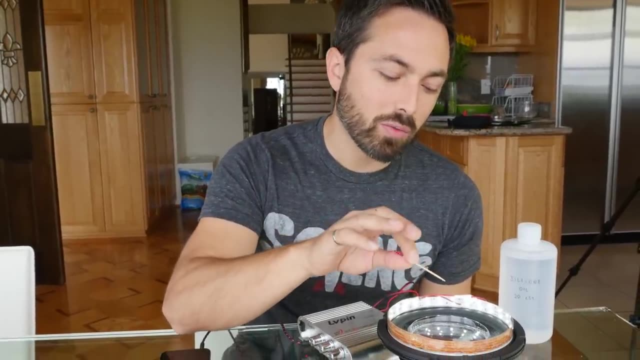 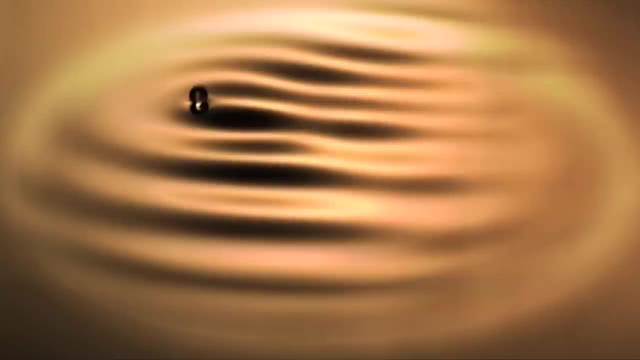 And the probability of the droplet crossing the barrier decreases exponentially with the increasing width of the barrier, just as in quantum tunneling. Perhaps the most surprising thing about these walkers is they exhibit quantization, just like electrons bound to atoms. Here the walker is confined to a circular corral. 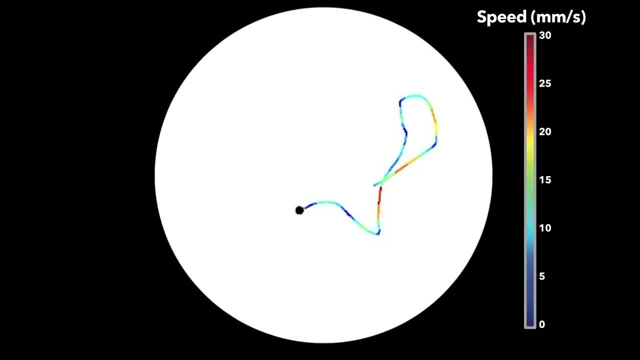 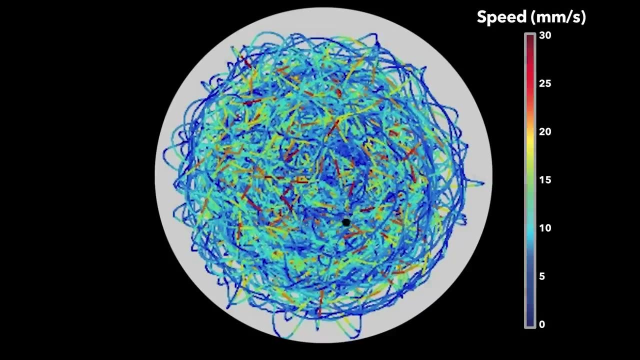 The droplet seems to move around randomly as it interacts with its pilot wave. The complex interaction between the droplet and the wave leads to chaotic motion of the droplet, But over time a pattern builds up. This is the probability density of finding the droplet at any point within the corral. 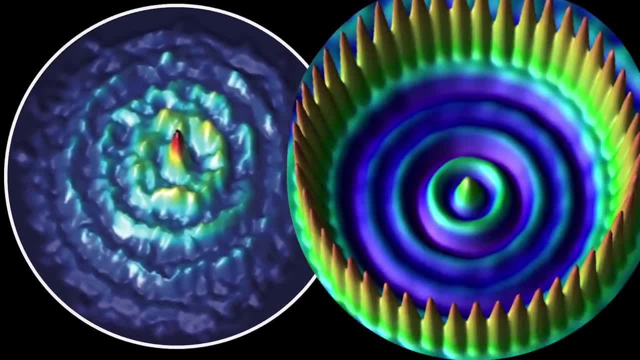 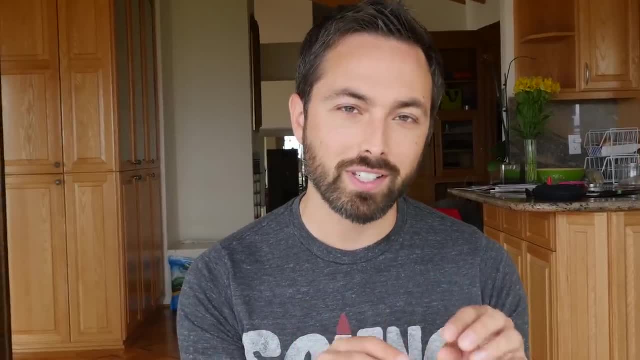 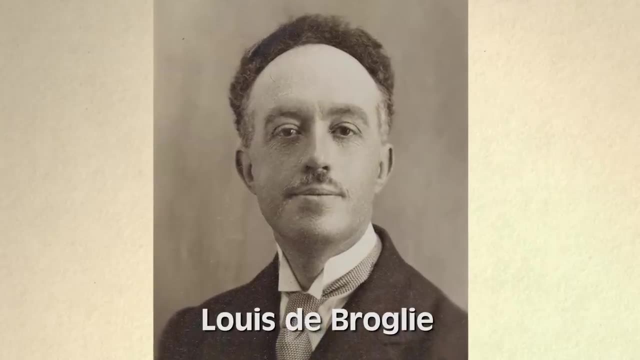 And it looks very similar to the probability density of electrons confined in a quantum corral. All of these similarities are no coincidence. The walking droplets actually create a remarkable physical realization of a theory proposed by de Broglie nearly a hundred years ago, in the early days of quantum mechanics. 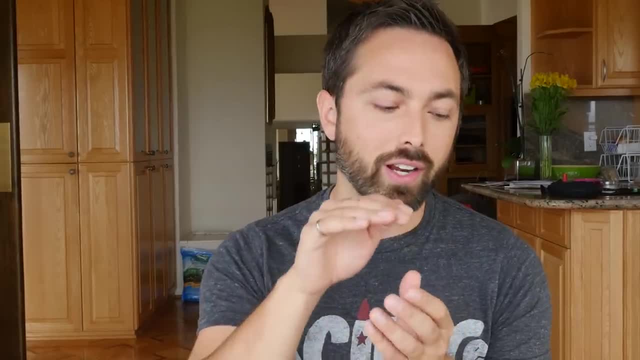 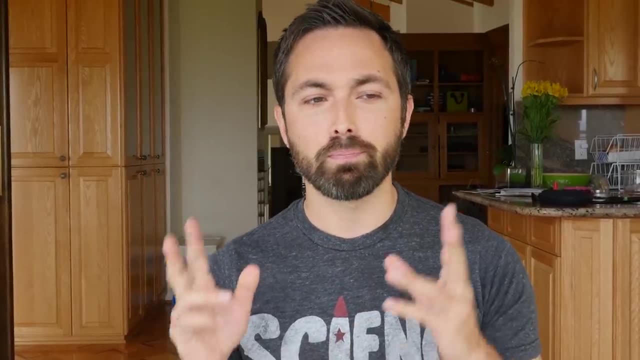 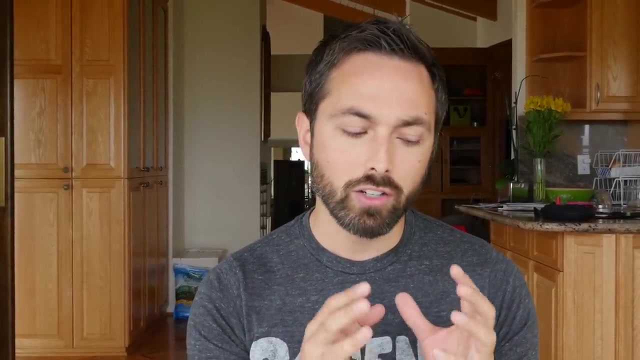 He postulated that all particles have a wave that accompanies them and guides their motion, And that wave is actually created by tiny oscillations of the particle. Now, this pilot wave theory was marginalized when the standard Copenhagen interpretation became widely adopted. The Copenhagen interpretation excludes anything that cannot be directly observed. 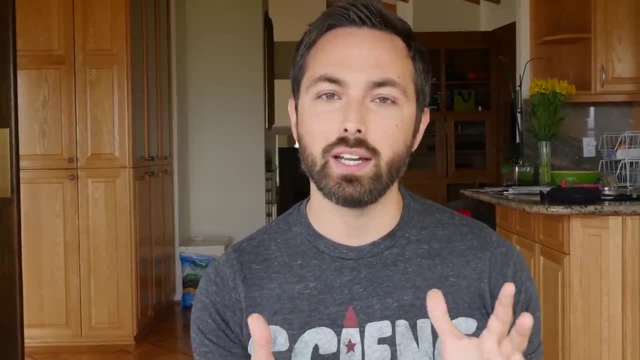 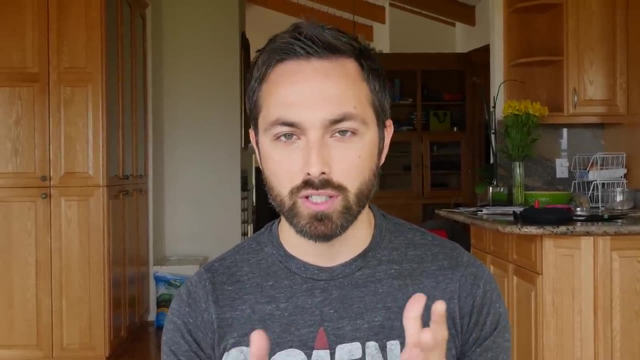 And it says everything that can be known about a particle is contained in its so-called wave function, But adopting this view forces you to give up on some common sense notions, like the idea that particles have a definite position and momentum, even when they're not being measured. 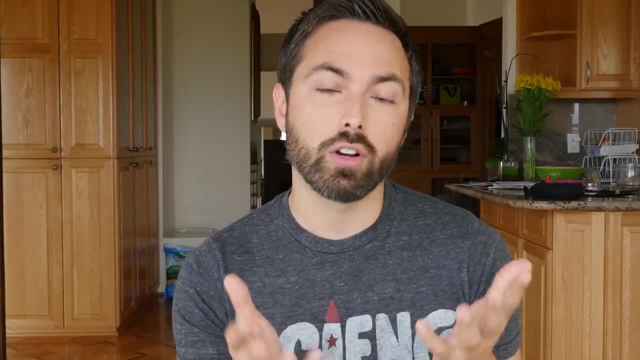 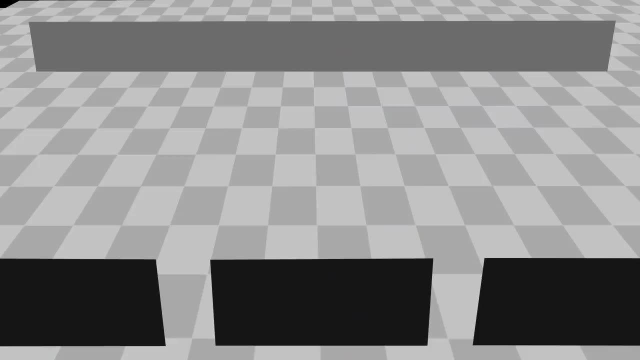 And it also meant that the universe was no longer deterministic. Randomness is built into standard quantum mechanics, For example. take the double slit experiment. According to quantum mechanics, the wave function of the electron is a superposition of the electron going through one slit. 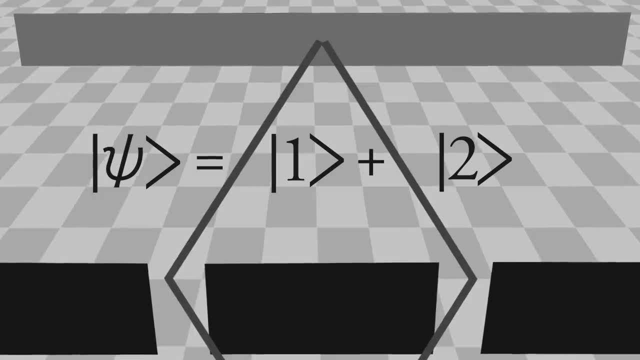 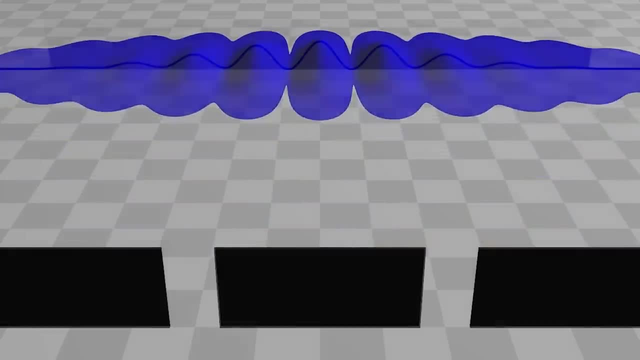 and the other slit simultaneously. Using this wave function, you can calculate the probability of where the electron is likely to be, And then, when you detect it at the screen, the electron pops up at one point at random that was in that distribution. 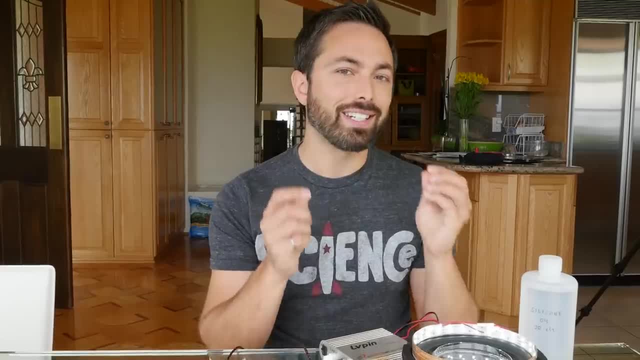 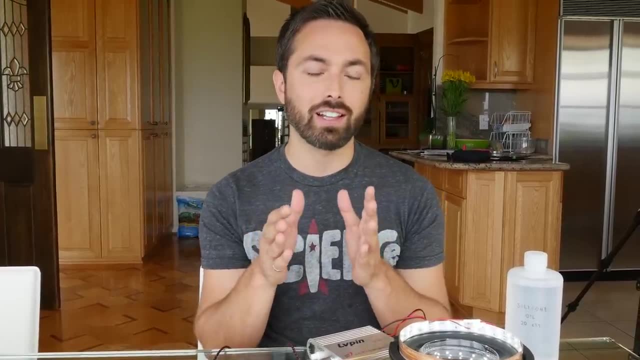 We say that its wave function collapses instantaneously at the moment of measurement. You can't say that the electron was there before you measured it, and you can't even say that the electron must have gone through one slit or the other. Compare that with the picture provided by the bouncing droplets. 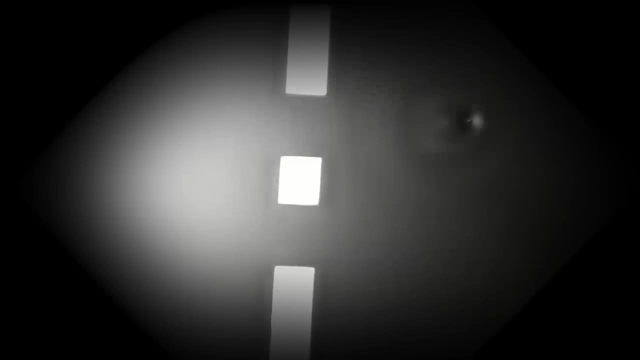 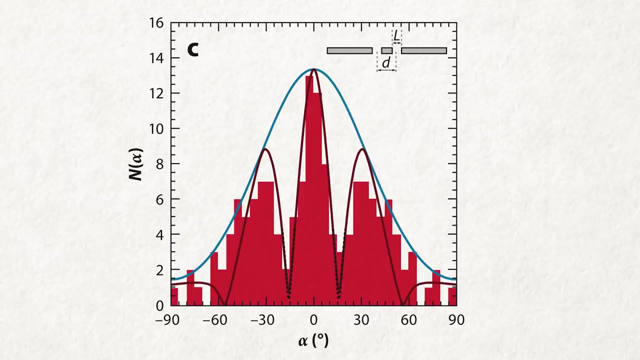 In this case, the pilot wave goes through both slits, but the droplet only goes through one. The droplet is pushed around by its interaction with the wave, so that the resulting statistical distribution is the same. The droplet never exists in two places at once. 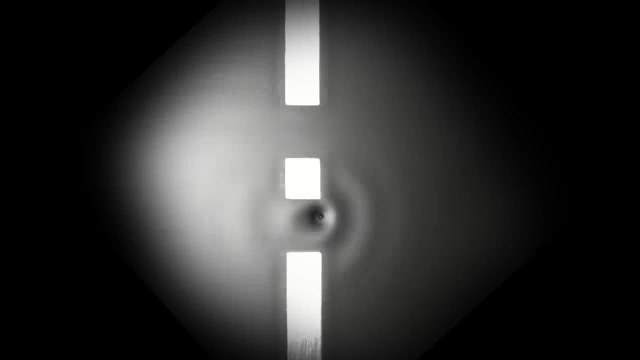 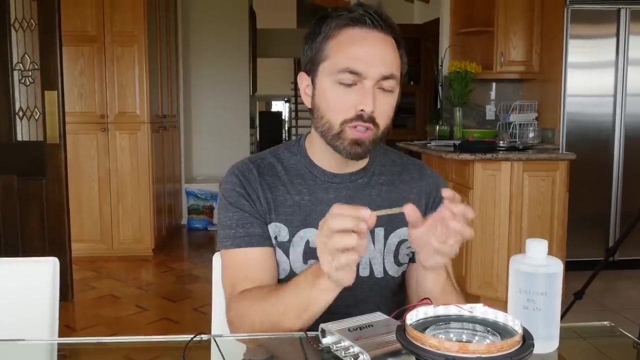 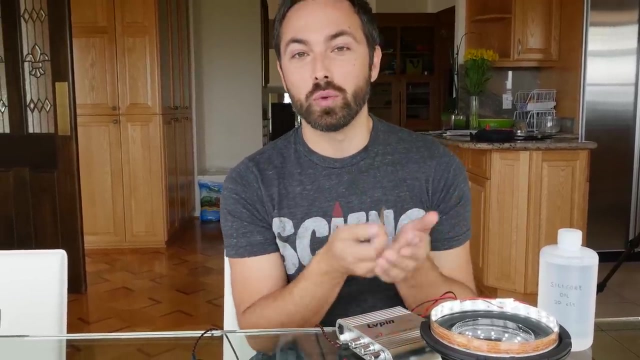 and there's no randomness. If there is any uncertainty, it's just due to our ignorance of what's going on. It's not that it doesn't exist. So pilot wave dynamics can produce many of the same results as quantum mechanics. Does this mean that this is really what quantum particles are doing? 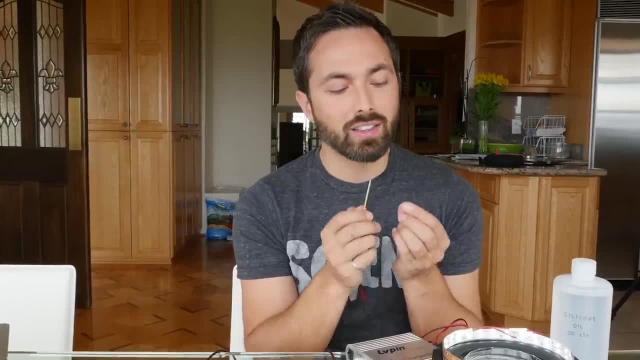 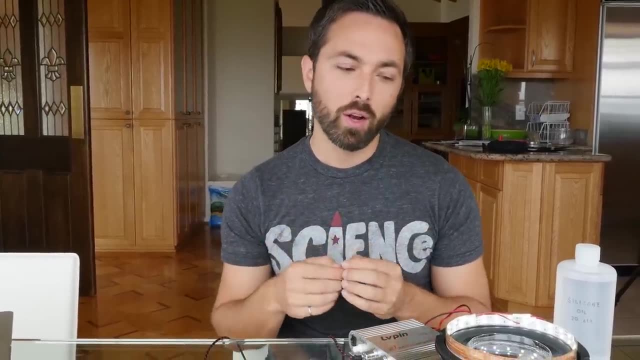 No, But I think it'll at least suggest that this is possible. These are possible dynamics that could lead to the statistics which are captured in the quantum mechanical theory, And what's appealing about this is it gives you a clear idea of what's going on. You don't have to abandon the idea that the universe is deterministic and you get particles with definite position and momenta. I think it's great that we have two competing theories for the same experiments And they both ask you to accept odd things, just different odd things. 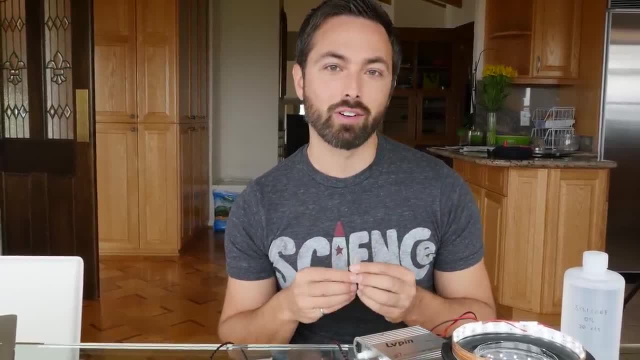 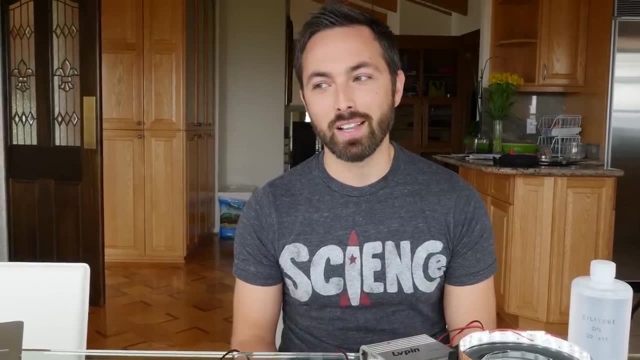 And it comes down to what you're comfortable with Really, whether you prefer the Copenhagen Interpretation of Standard Quantum Mechanics or a pilot wave theory. Let me know what you think in the comments. Do you like the pilot waves? I mean? it's definitely a very appealing picture.